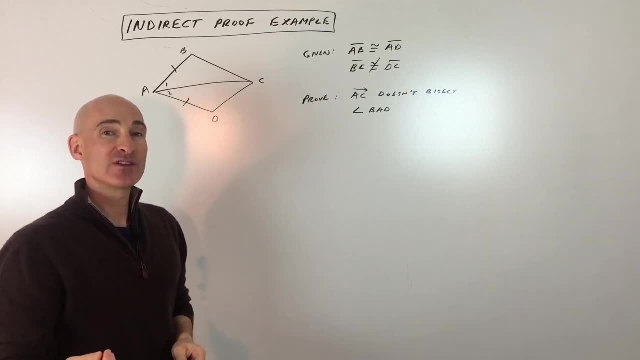 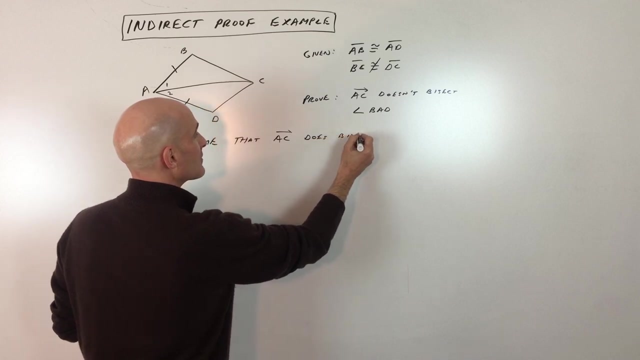 take what you're trying to prove and temporarily assume that the opposite is true. Okay, so do you understand? So you take what you're trying to prove and you temporarily assume that the opposite is true. So I'm just going to write this down. So let's just assume, okay, temporarily, that AC- okay, we'll just say ray, AC- does bisect angle BAD. Okay, so you with me so far. So that's. 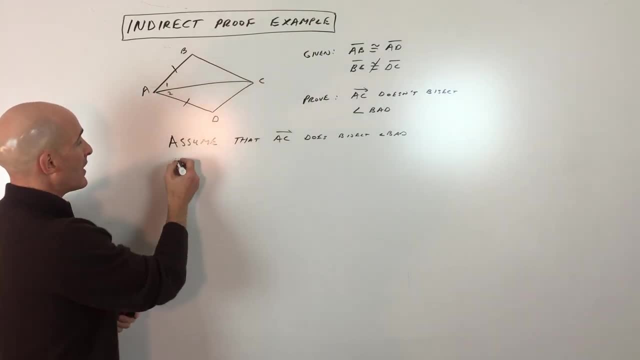 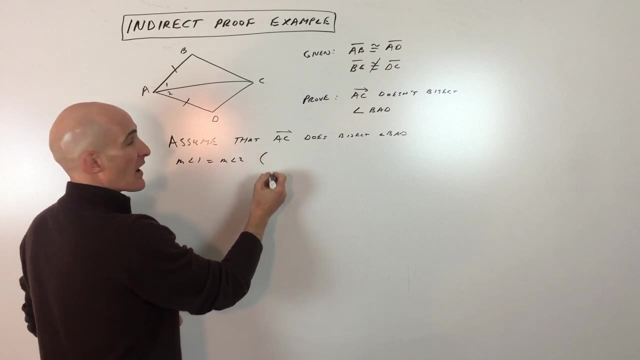 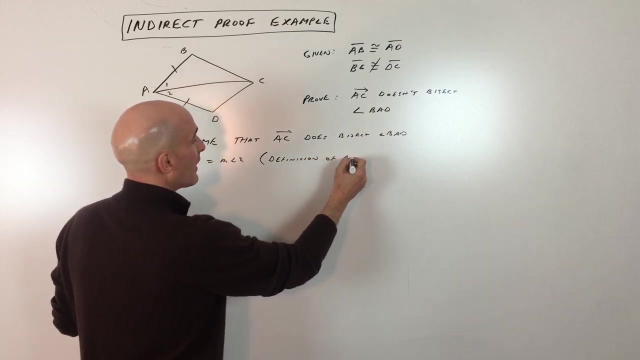 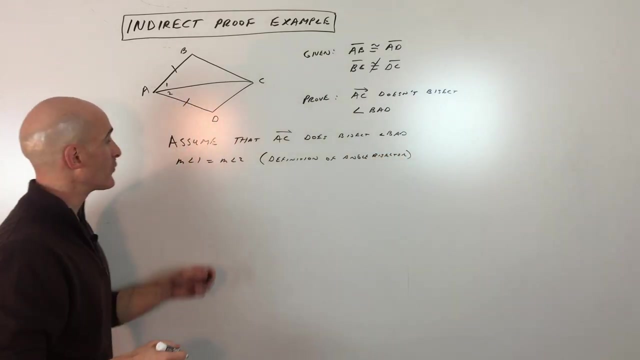 if we assume this does bisect, then we know that the measure of angle one is equal to the measure of angle two, And that's by the definition of an angle bisector. So definition of angle bisector. So this is more of like a paragraph type proof as opposed to a two column proof. So now we know that angle one is congruent to angle two. So I'm just going to mark that on our diagram And we also 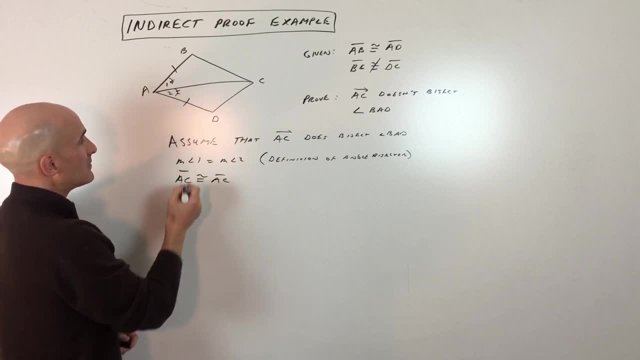 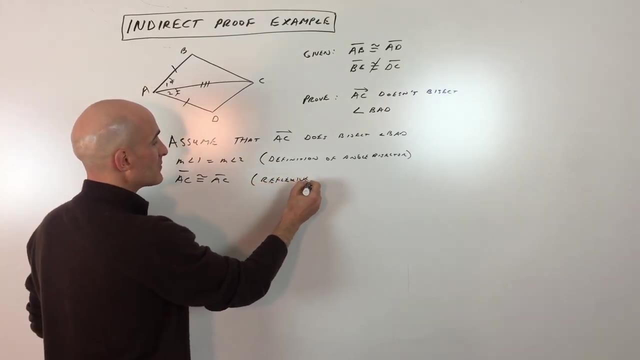 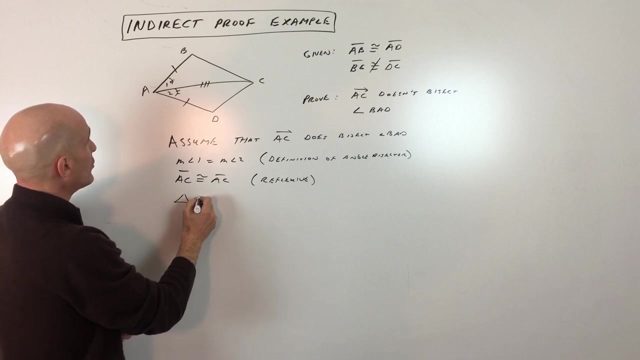 know that AC is congruent to AC. Okay, it's congruent to itself, And that's by. I'll just put in parentheses here: reflexive property, right, reflexive anything is congruent to itself, And so what you notice here is that this triangle and this triangle are congruent, So this is triangle. 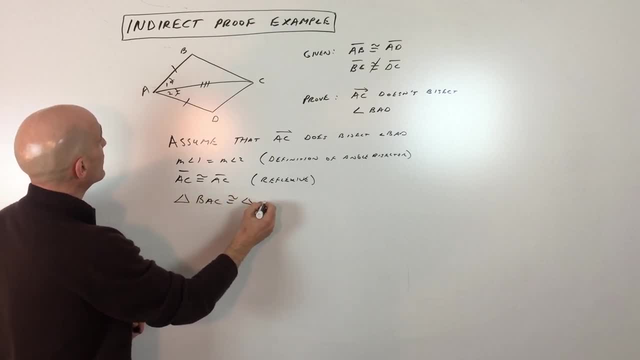 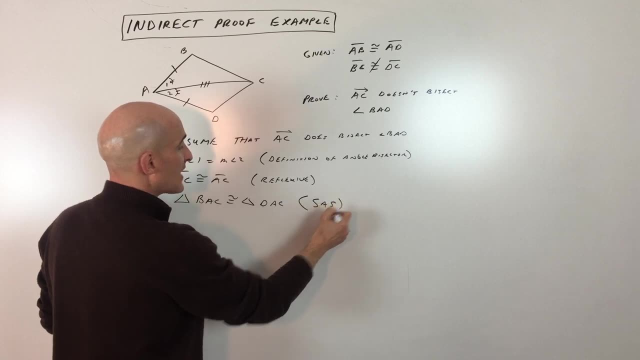 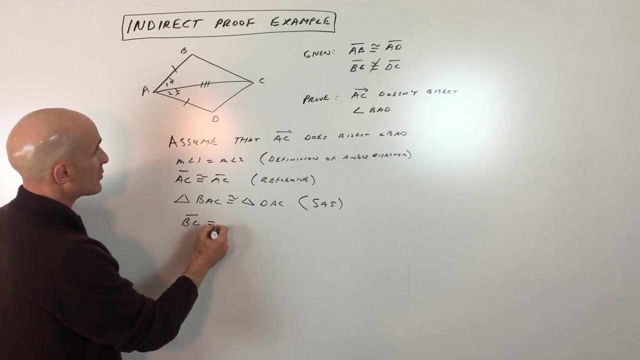 BAC is congruent to triangle DAC And the reason would be by the side angle side, Okay, side angle side. So now we know that these two triangles are congruent, we can say that BC is congruent to DC And that's. 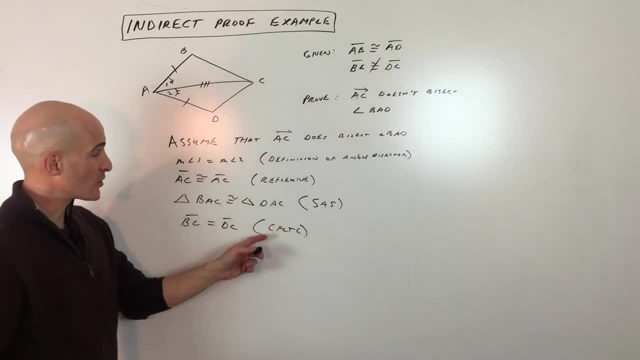 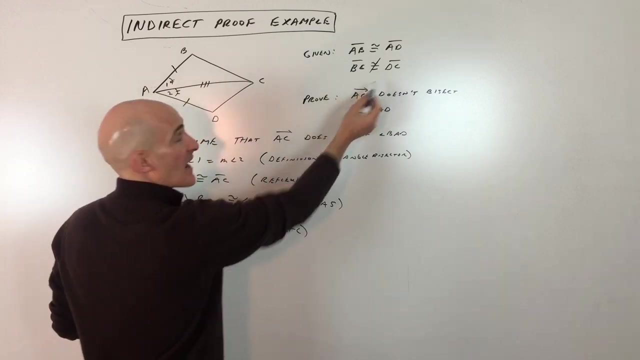 by the CPCTC, which means that the corresponding parts of congruent triangles are congruent. Once we prove these two triangles are congruent, the parts that match up, meaning BC and DC, will also be congruent. Okay, however, what do we notice here? However, this is a contradiction of one of 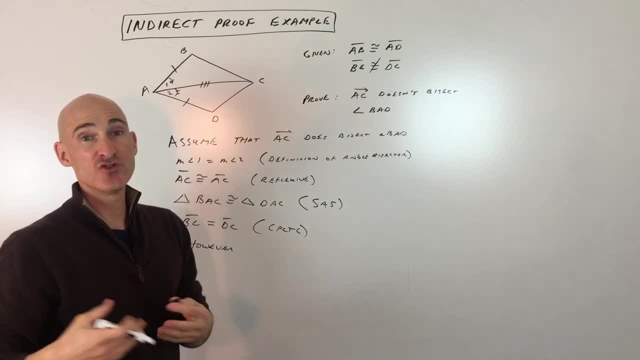 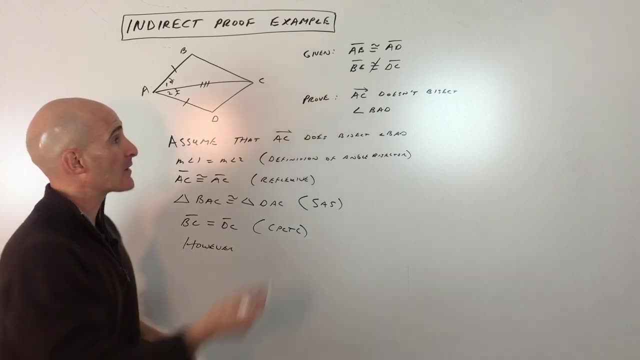 the givens. So whenever you get a contradiction of a given or something that you know, that is true like all the angles in a triangle led up to 180, or you know, parallel lines don't intersect or a known fact or one of the givens.